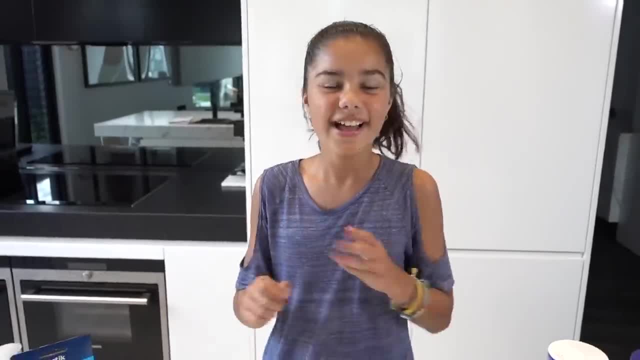 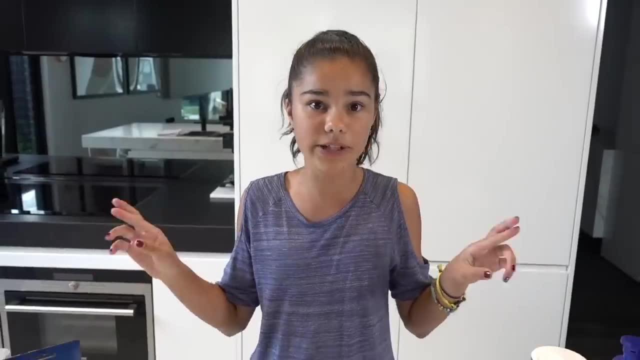 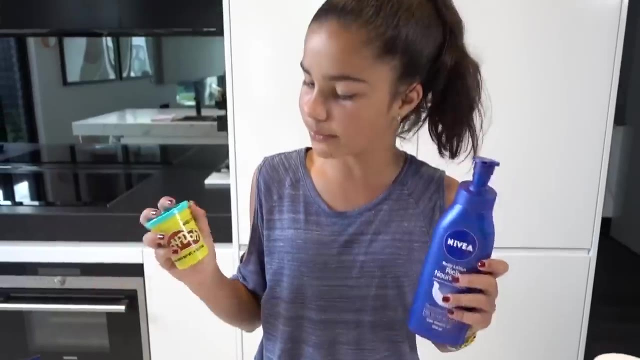 contain no glue at all. So here I have some different ingredients and notice that they contain no glue or borax. So I'm really hoping that these ones work. So let's start with the first one. So here I have some Play-Doh and some lotion, and this is called Play-Doh. 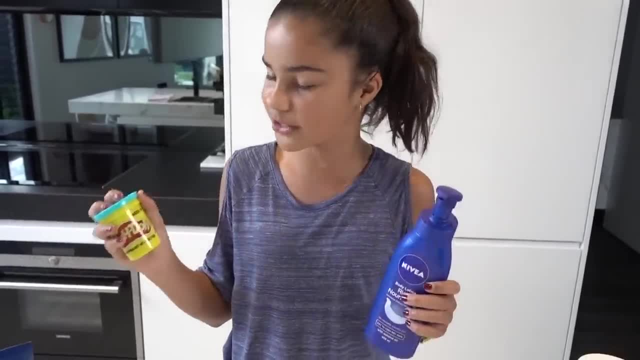 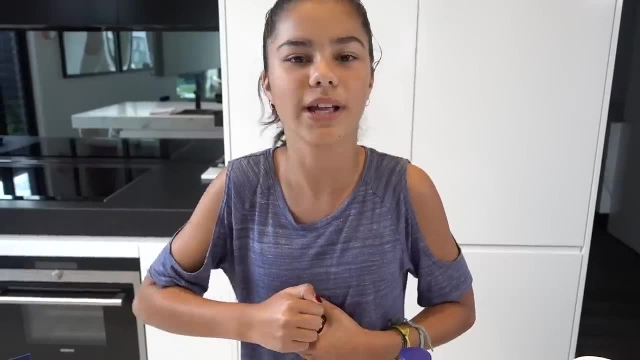 slime. So apparently if I mix lotion with this Play-Doh it's supposed to make it soft and stretchy. So today we are going to find out if it does. Here I have some quite like old Play-Doh that has been used before. I'm sure James won't mind if I use it. It's a. 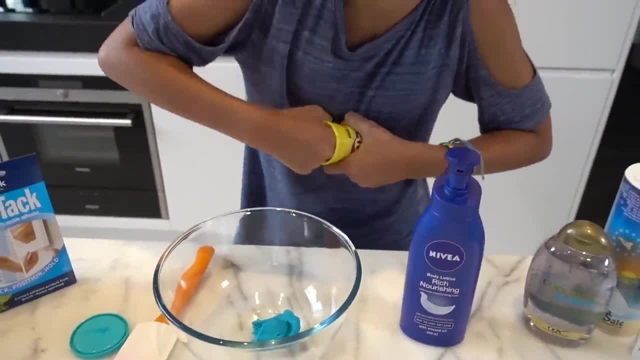 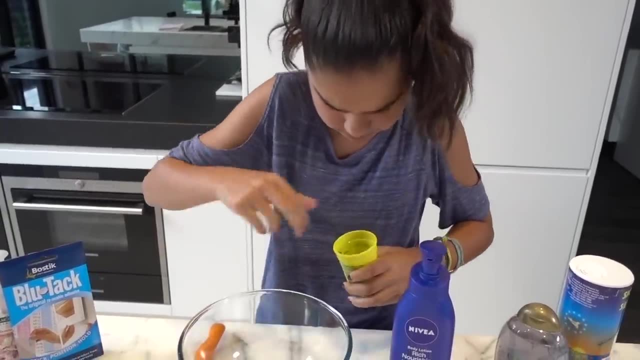 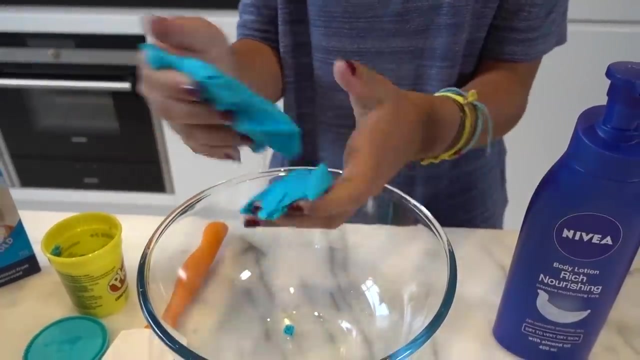 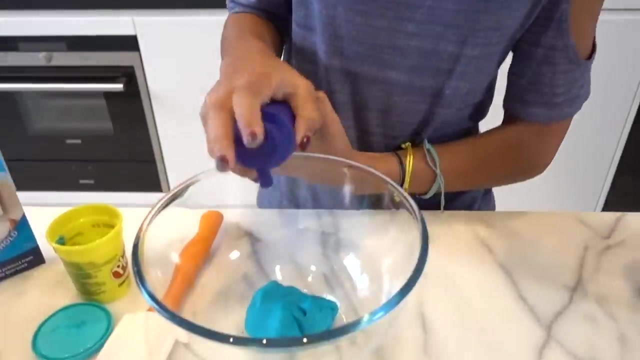 really nice colour. Oh, it's a bit hard to get out, though. Come on, Alright, that should be fine. It's really soft already, but it's not notice, it's not very stretchy. So now I'm going to try and add some lotion to this slime. I'm going to 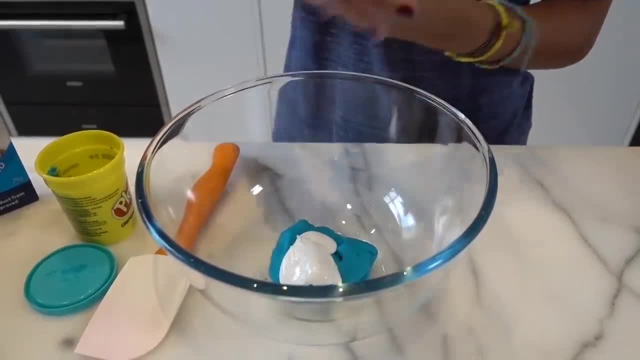 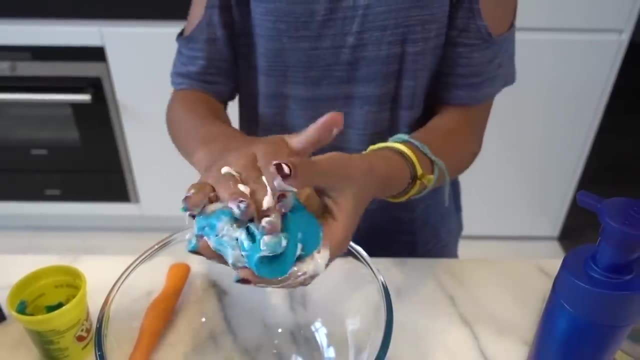 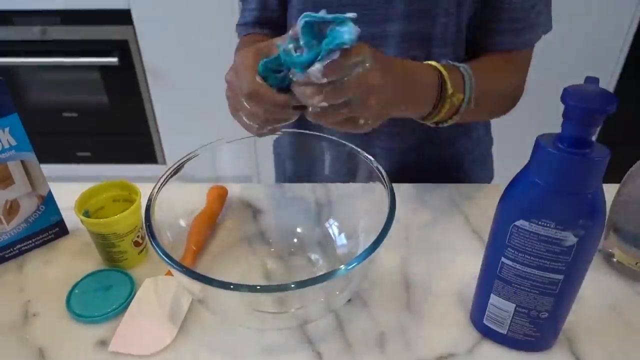 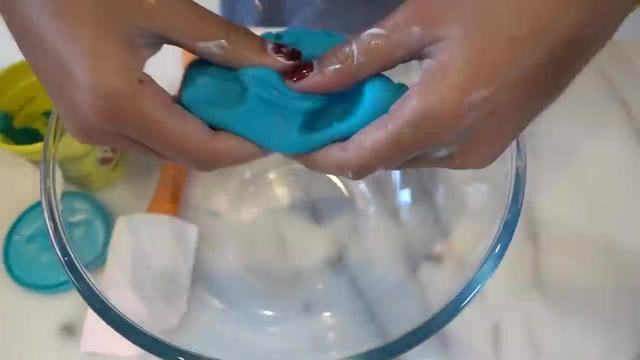 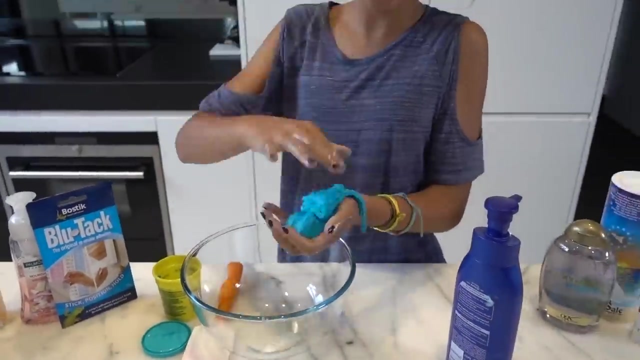 add a couple of pumps. Now I'm going to knead it through and let's see if it makes some nice slime. It's a bit hard to knead in, so this might take a while. Ok guys, as you can tell, that took a lot of kneading and a lot of lotion, more than I expected. 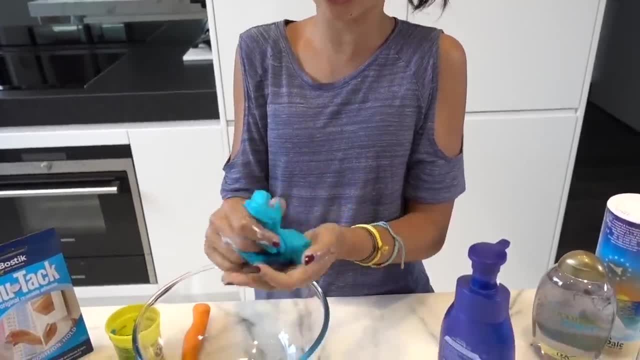 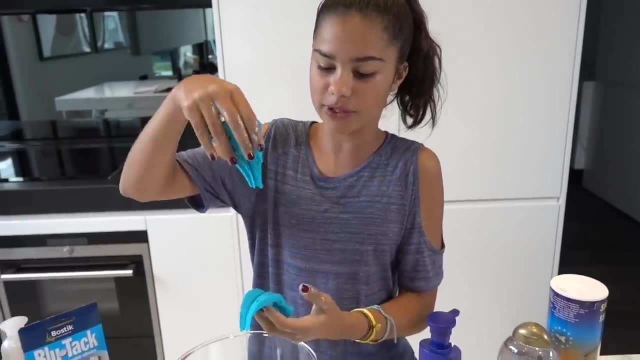 And it's gotten to a really good consistency. actually It's so super-duper soft, But I found that it's not that stretchy. I saw that it's supposed to be stretchy after you add in the lotion, but mine's not really. 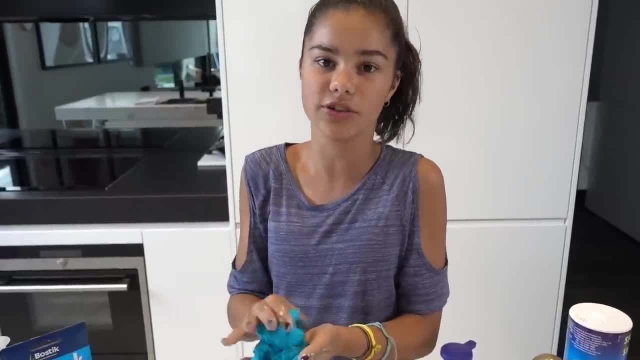 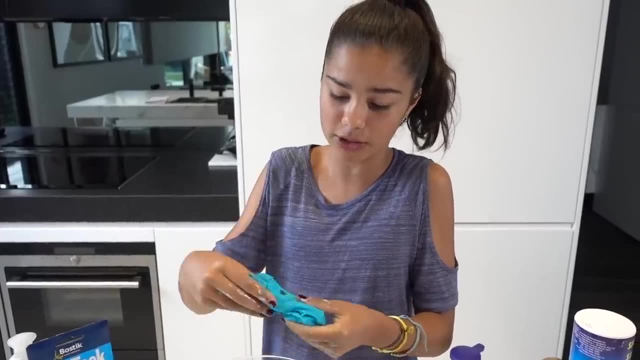 working that much with the stretchiness, so maybe I need to use a different lotion or something. I'm not doing it right, but it's pretty good. I will say that this one worked because it is a pretty good consistency. it has a nice 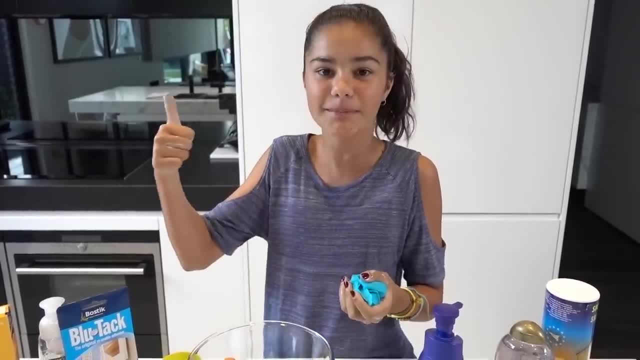 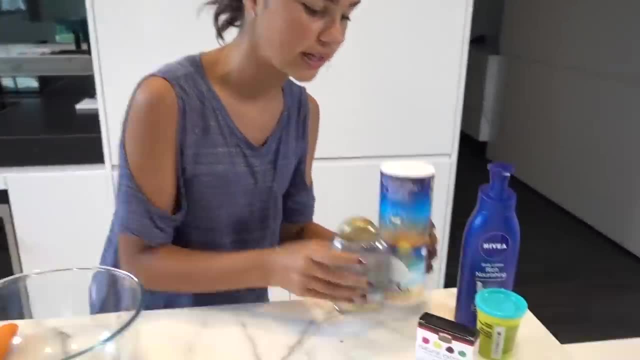 texture, and it's very soft as well, so I'm going to give this one a thumbs up. Let's move on to the next one, All right guys? so the next slime that I'm going to be trying is shampoo and salt slime. 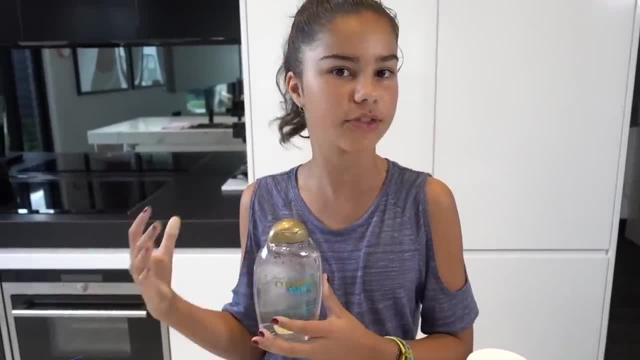 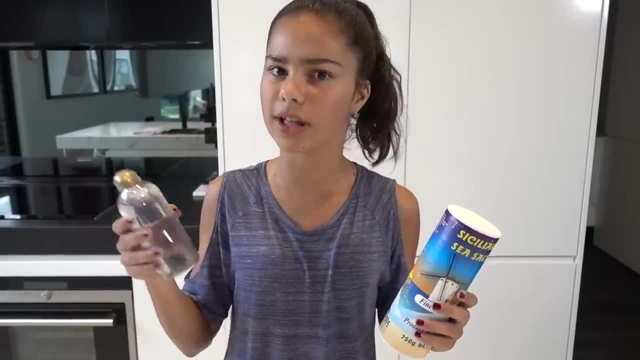 So it's been recommended to use a gel shampoo because it's really thick and apparently, when I pour some of this into the bowl, I'm supposed to add a thin layer of salt on top, and then it's supposed to clump up and then I'm supposed to put it in the freezer for. 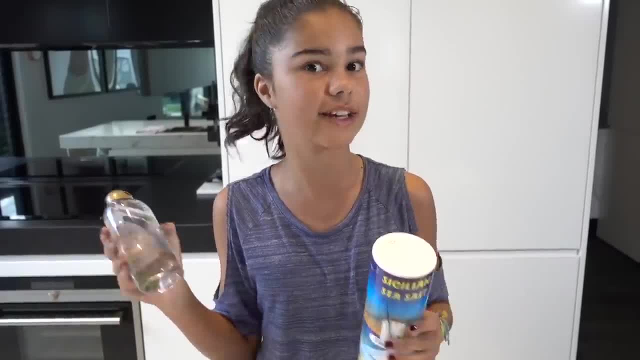 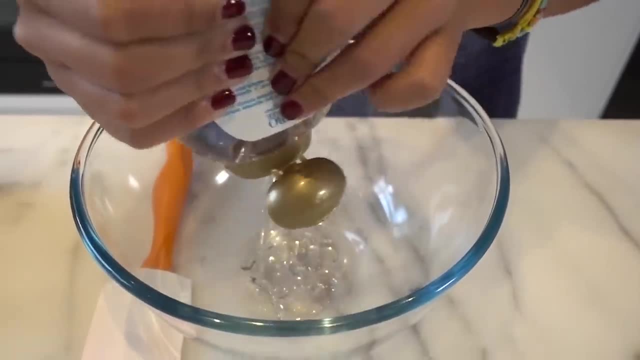 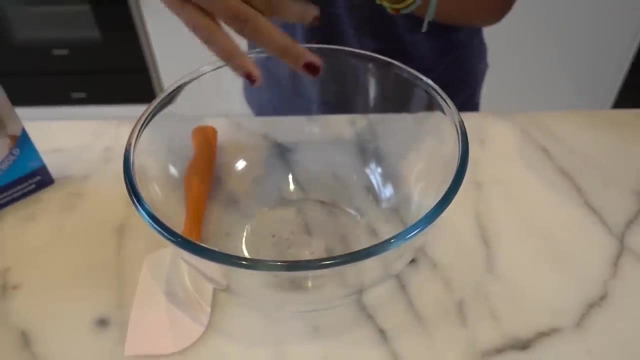 10 minutes and then it will turn into slime. So let's see if this one works. First thing, I'm just going to pour in not too much of this here shampoo, or maybe a little bit more. That's fine. And next I'm going to be adding in some food coloring to make it nice and pretty. 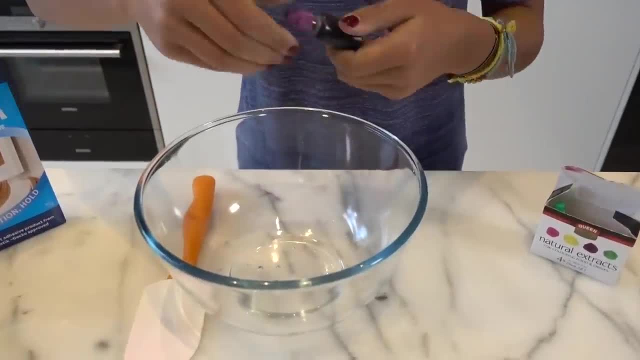 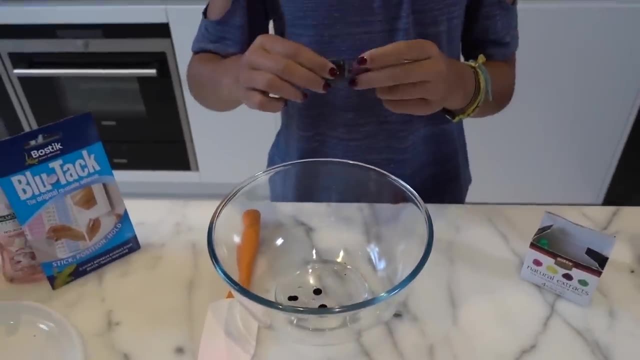 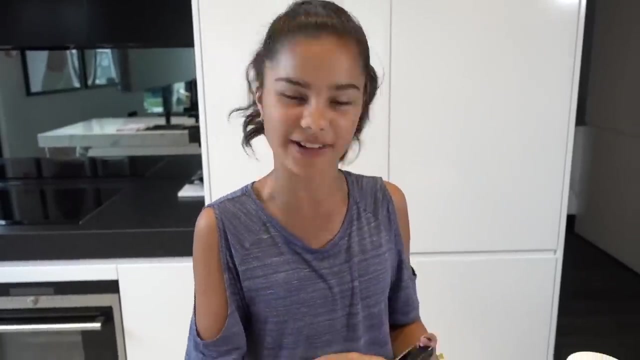 I'm going to be using purple and I'm just going to add a couple of drops of this And may I say this shampoo smells so good. it smells like pineapples and coconuts. I guess it is coconut water. 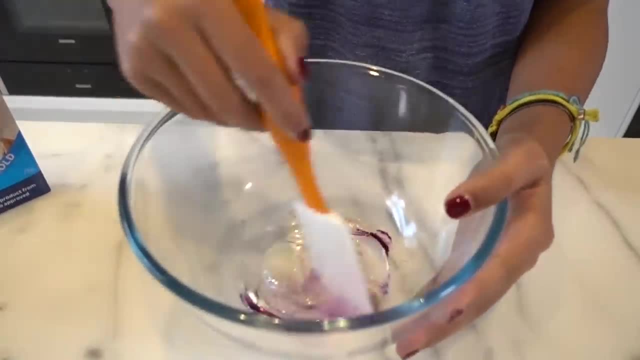 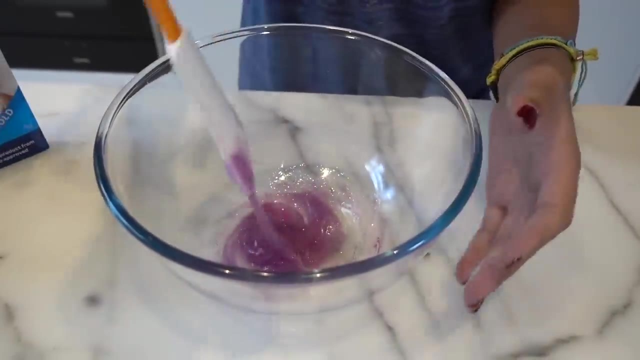 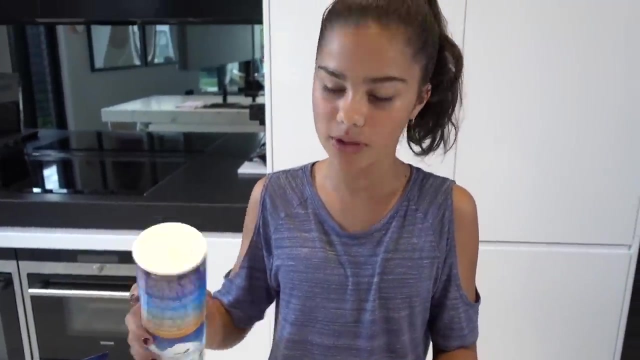 And I'm just going to give that a stir. It's so thick, guys, All right, And now I'm just going to add a thin layer of salt on top. This is just like table salt, so I don't want it to be too crystal-y, the salt. 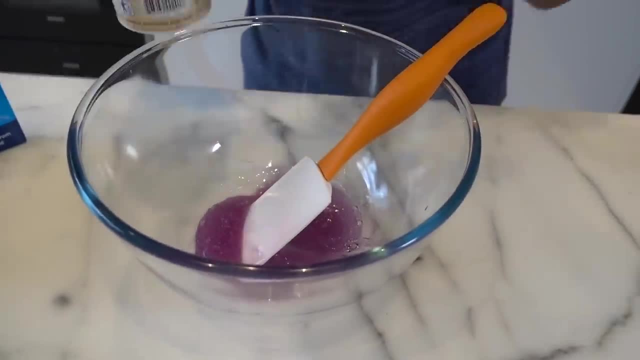 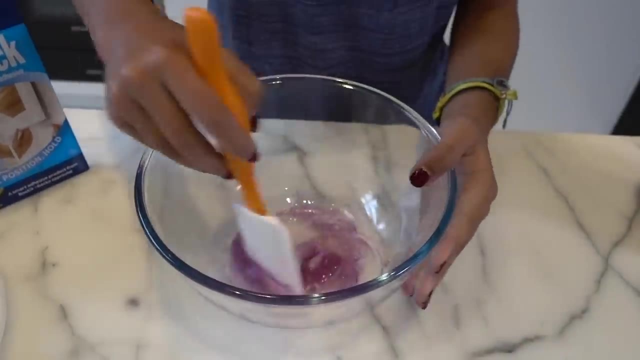 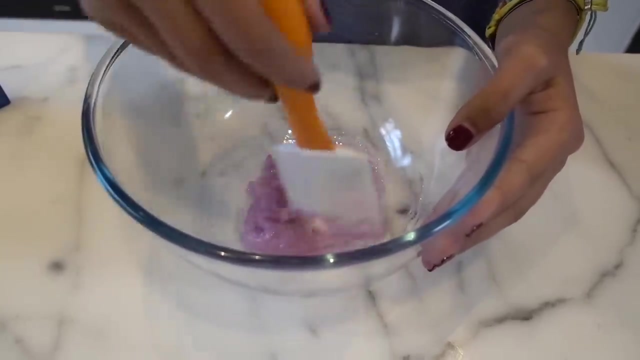 All right, that should be enough. Hopefully it's not too much. All right, And as you guys can tell, it kind of looks like it's starting to clump a bit together, like it's almost starting to activate. Now I'm not going to add in any more, because they only told me to add in like a little. 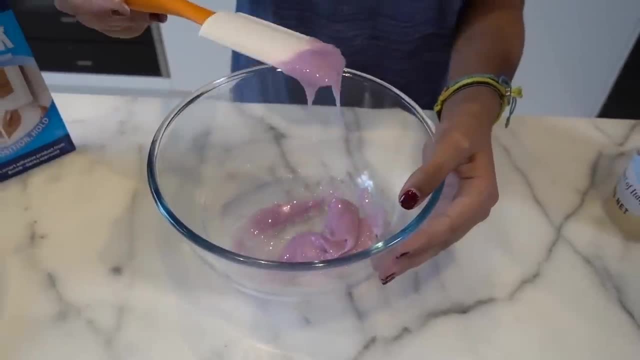 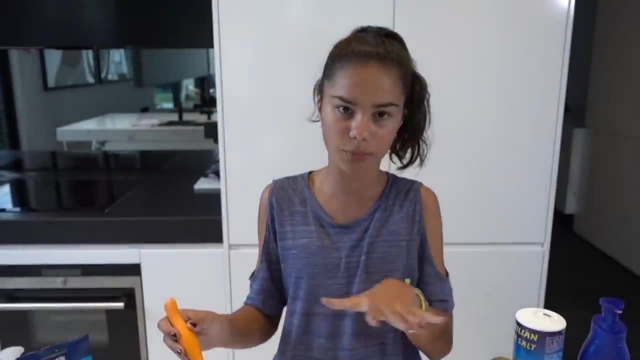 bit, or this recipe says to, so I think that's enough. Hopefully it's not too liquid. Now I'm just going to pour this onto a plate so it spreads out and it'll be easier for it when it freezes in the freezer. 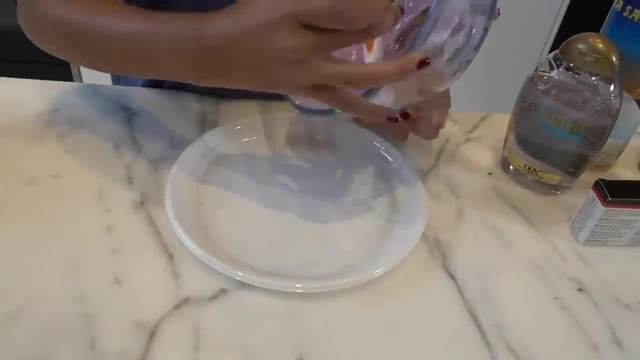 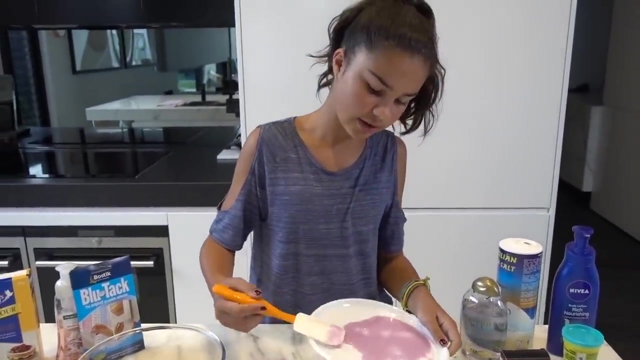 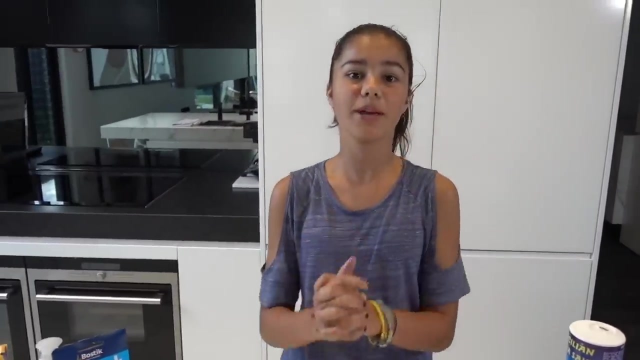 All right, I'm just going to give that a stir. All right, Let that spread out a little bit. and now I'm going to leave it in the freezer for 10 minutes. And now we wait. Maybe I should clean up. 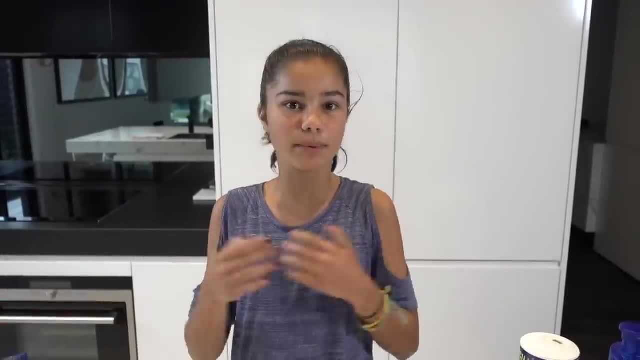 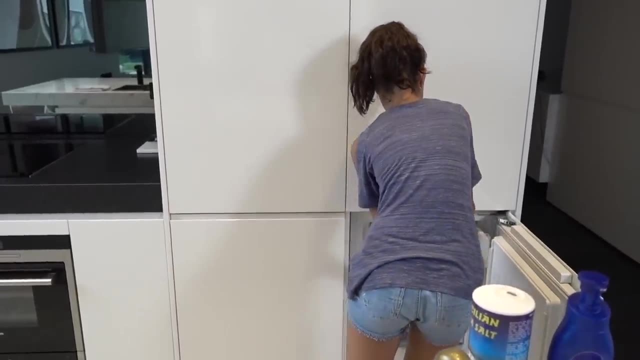 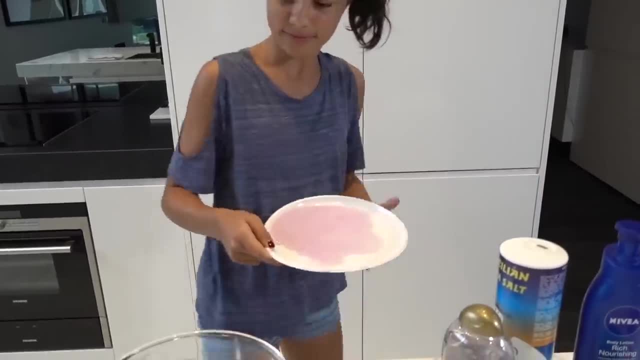 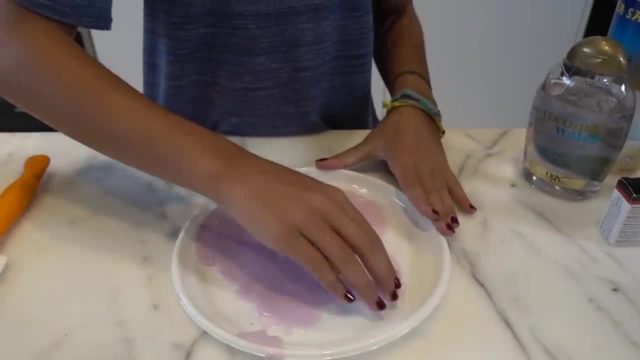 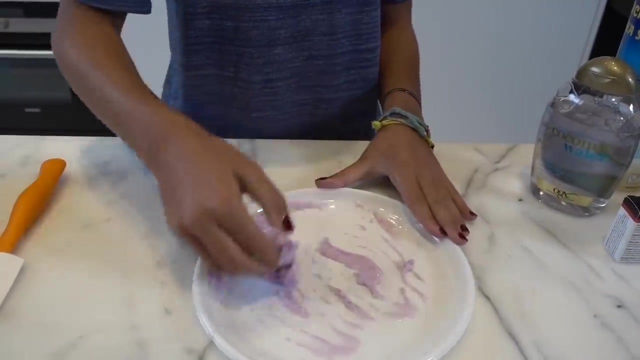 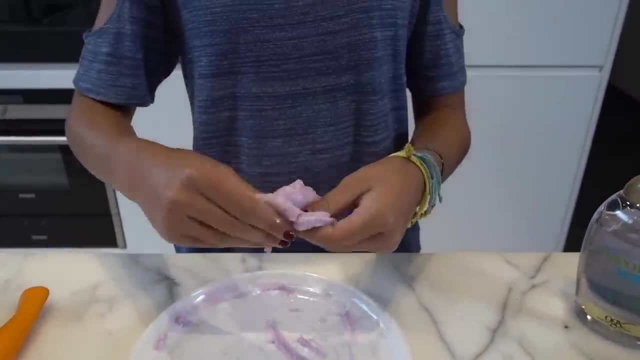 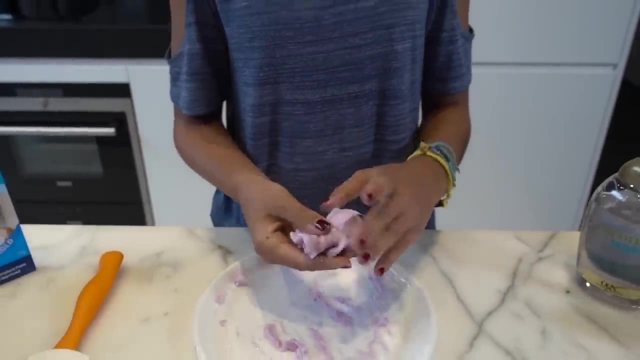 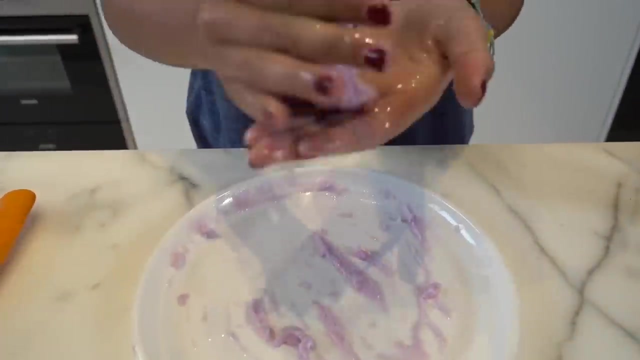 It's so cold. Now, guys, this again is really cold. Actually, you guys, it's kind of turned into slime, I mean like a very oily slime, But it's done something there stretchy. but I honestly, guys, I can't play with it. it's too cold. we've got to. 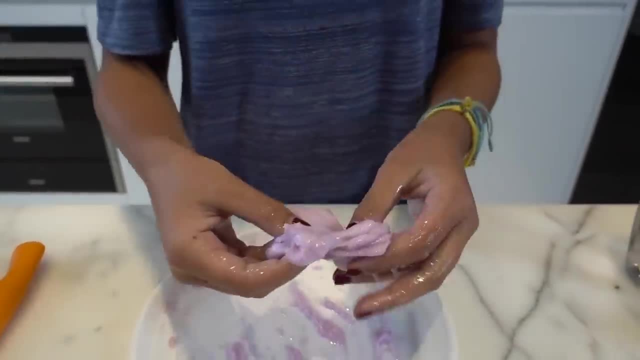 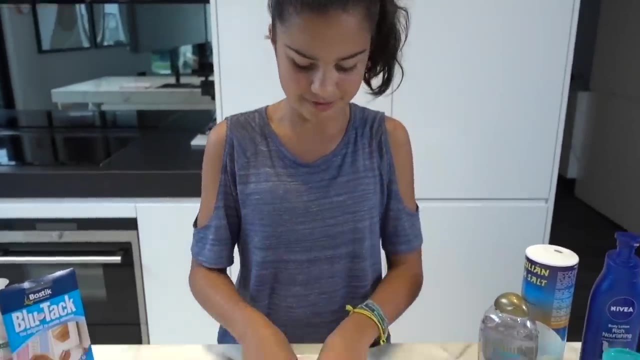 let it cool down, but I mean, it's not really like that really nice slime. maybe I didn't do it right and there's something else I need to do to it. yeah, it's not very good and it's freezing my hands off, so I'm not too sure about this. 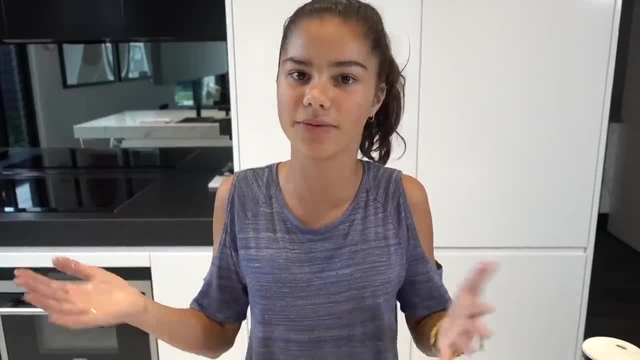 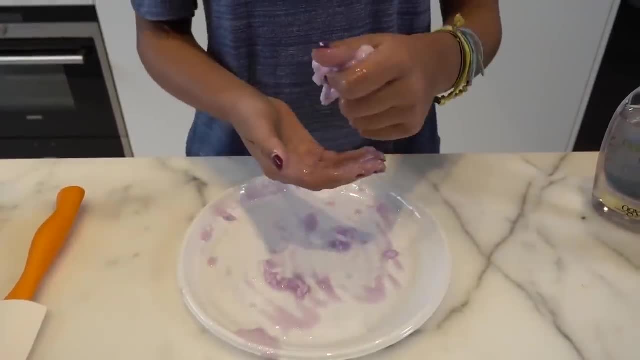 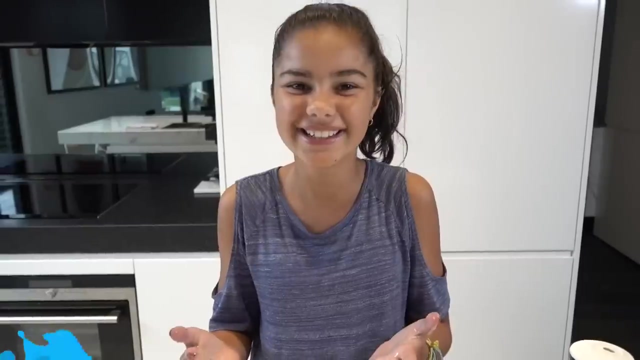 slime it can. you got like you guys can maybe comment down below how to make this one work, because I'm not too sure about this one. all right, let's move on to the next one, and I think I need my hands in my boiling water. I'm gonna numb. 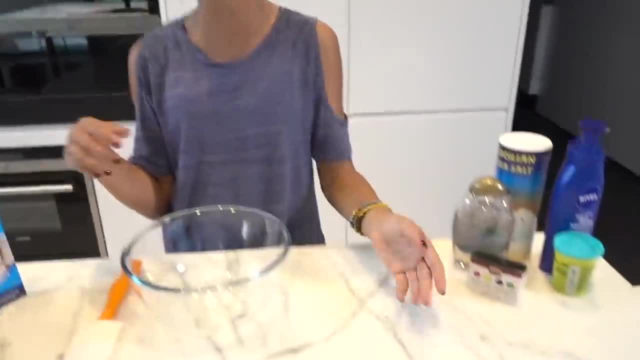 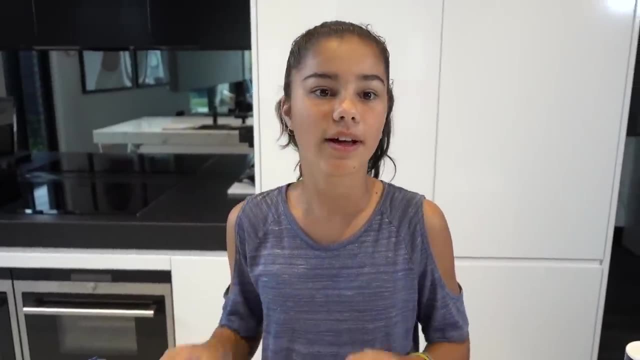 well, guys, I am a little bit disappointed that the last one didn't work. as you guys can tell, it is now look good, not even slime anymore. but I wonder if I did something wrong. hopefully you guys can tell me if I did you something wrong, because I actually have seen. 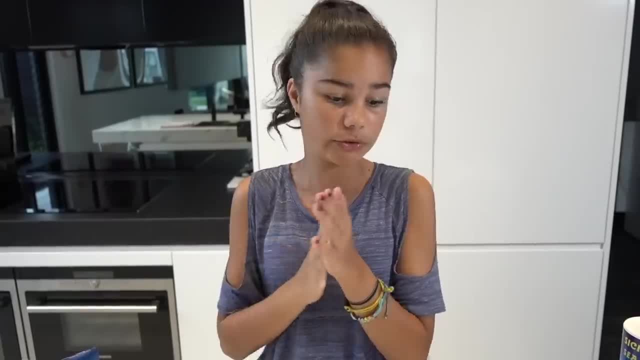 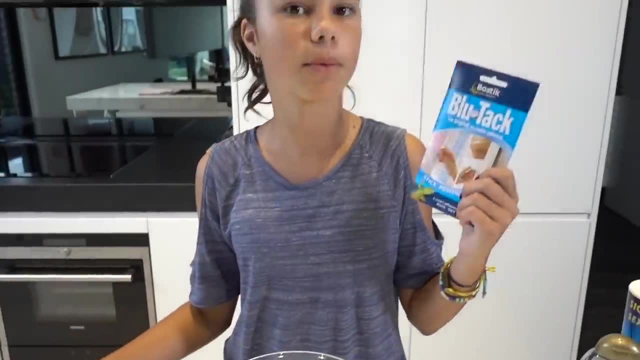 other ready прош tears road. well, that's why I wanted to add a lime. recipes that have worked before, so I'm not sure what's happening there anyway. so the next time that I'm going to be trying is blue tech slime. so supposedly when I add some foaming hand soap to some blue tech, it will turn nice and 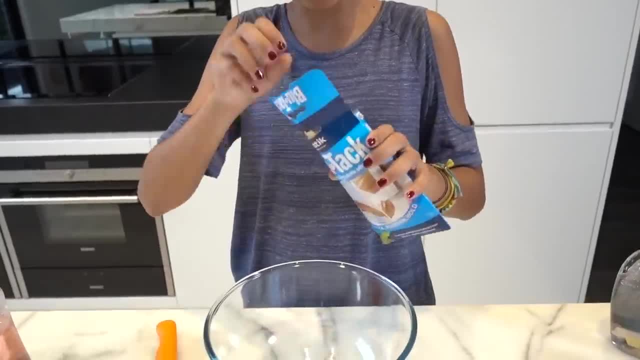 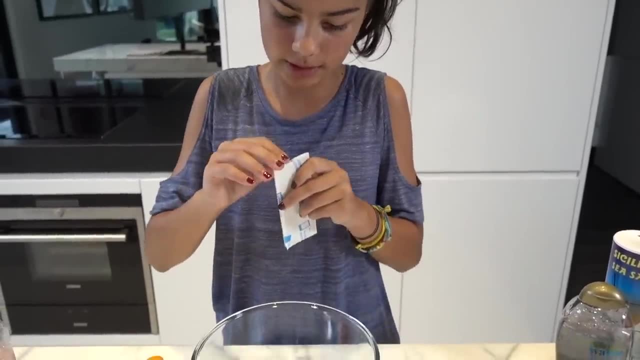 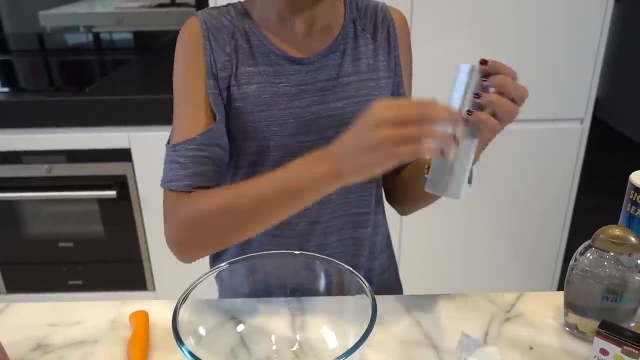 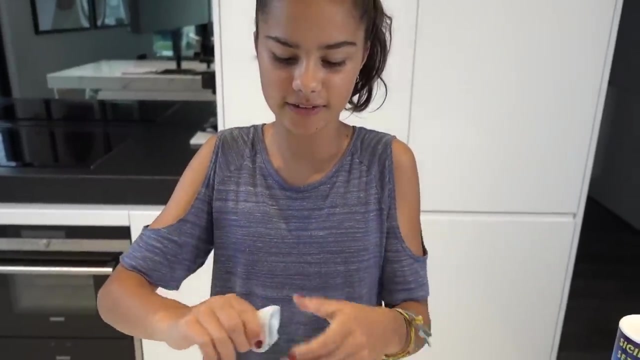 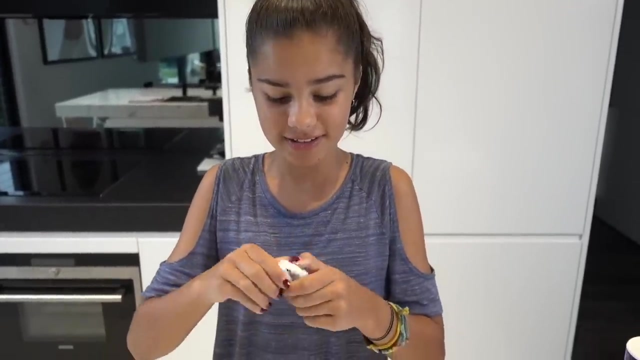 soft and stretchy. so let's try. I'm just gonna be using a couple of strips, maybe I'll do two. let's open it up. here we go. wow, I'm just going to quickly mix it together to make one slime. as you guys can tell, it's very rubbery, supposedly stretchy. 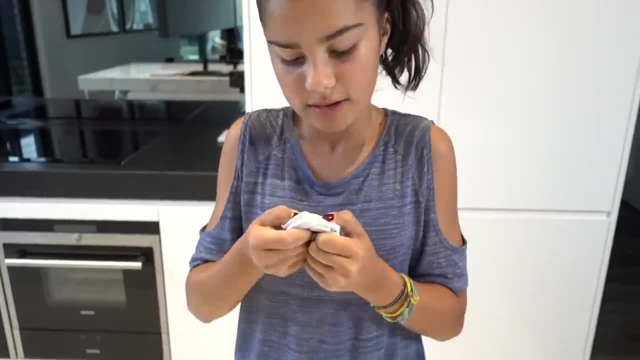 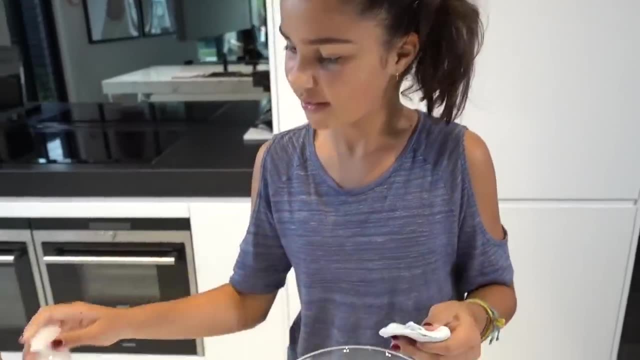 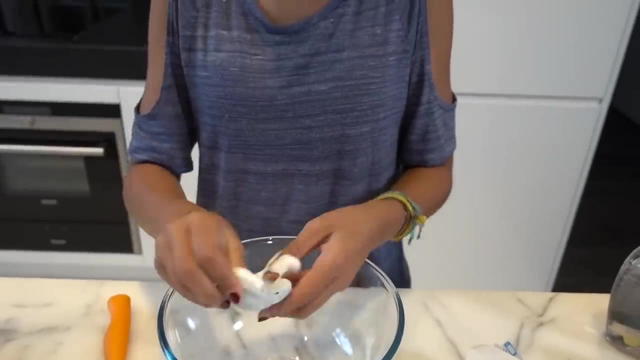 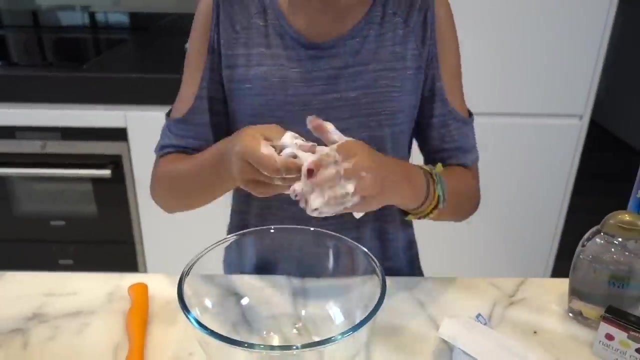 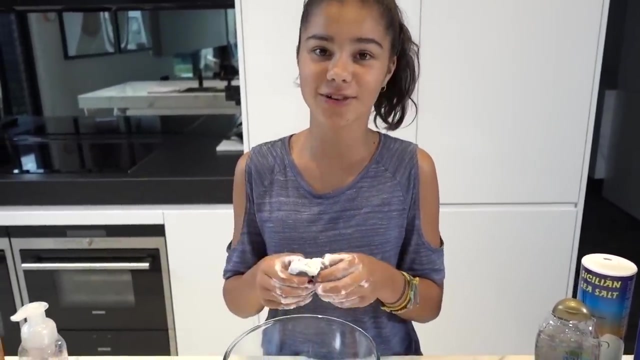 and now I'm going to to be adding in some foaming hand soap to this. It is very hard. I'll just do maybe two pumps And let's start. Guys, this is actually a real arm workout. It is so hard to try and mix in, but I'm determined to keep on trying. 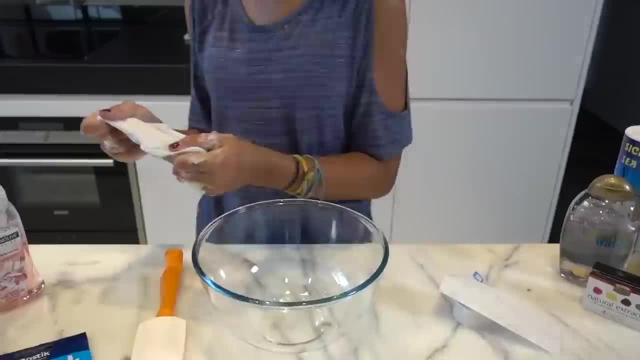 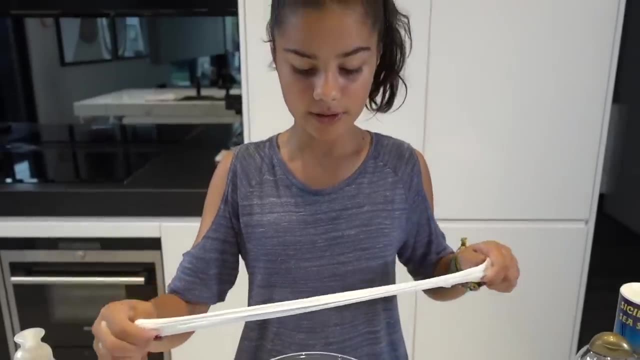 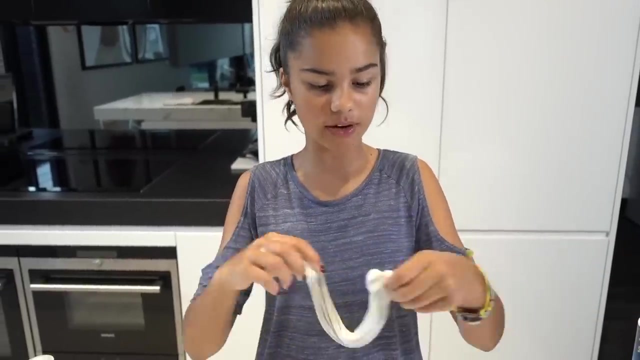 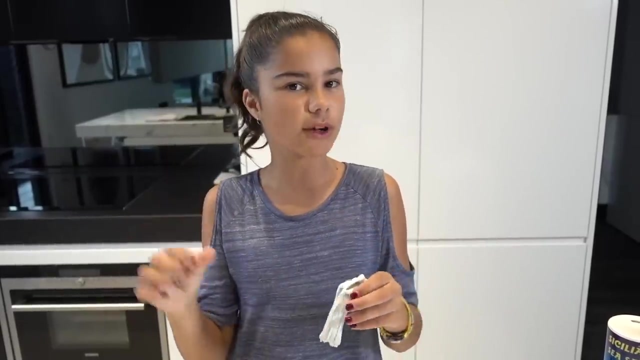 So, guys, after a little bit of kneading- actually a lot of kneading- this one did actually seem to work out. It feels a lot softer and actually much stretchier, much easier to stretch. It's not very rubbery, but to make it just a little bit softer, I want to see what happens when. 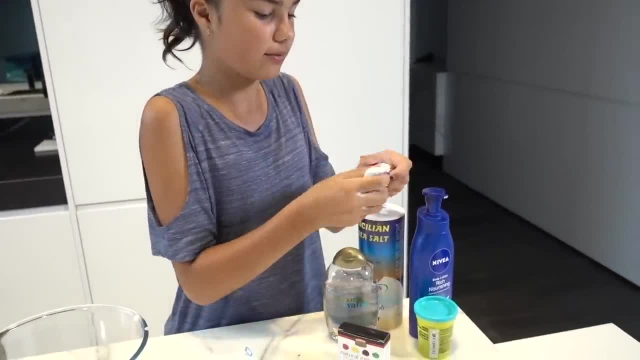 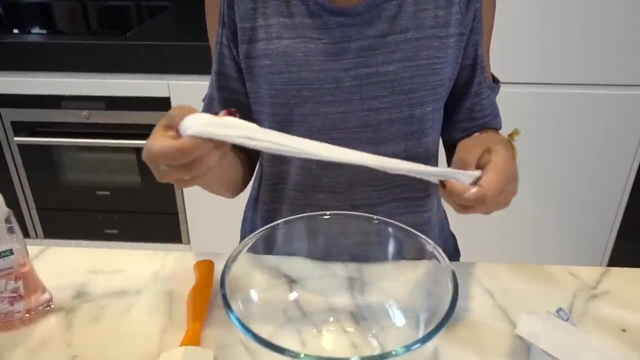 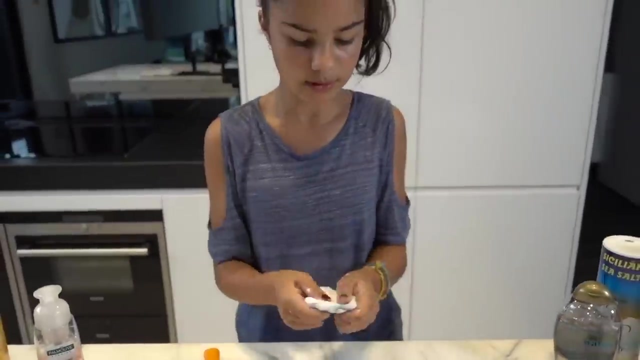 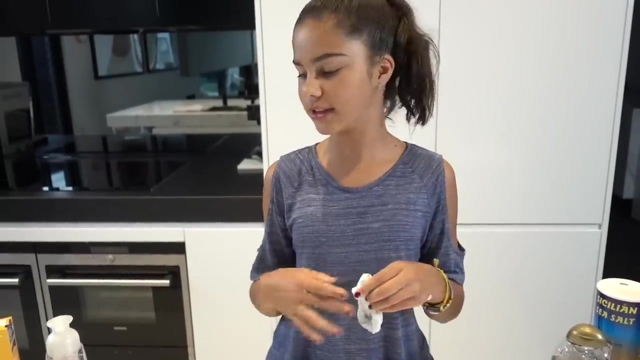 I add in a little bit of lotion. Hopefully it doesn't wreck it. I think one pump's enough. Let's see what happens. Alright, guys, after adding a little bit of lotion in it did kind of feel a little bit better, maybe a bit softer, but honestly you don't really need to add in that, But it actually. 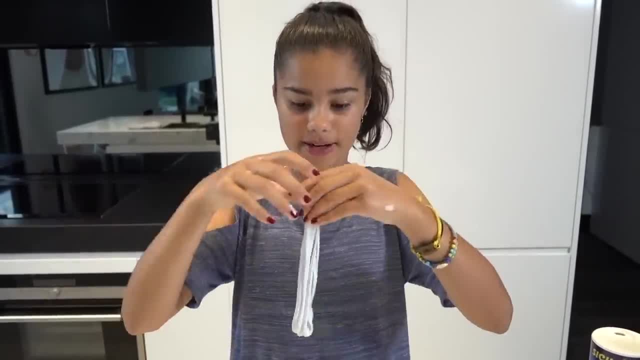 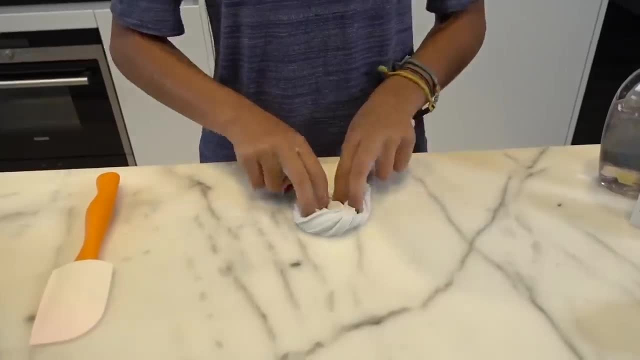 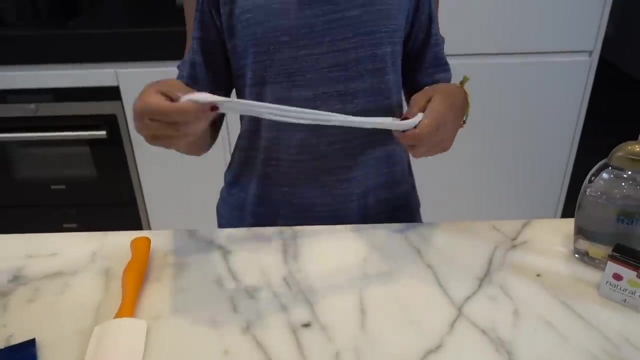 did work and made a really soft and actually very stretchy slime, And I really like this one. I'm going to give it a big thumbs up. Let's do a little swirl. It's not very good with pokes, though. Oh, it's pretty good actually. I like this one. 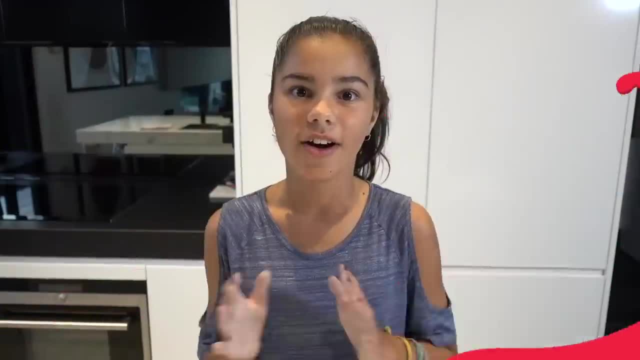 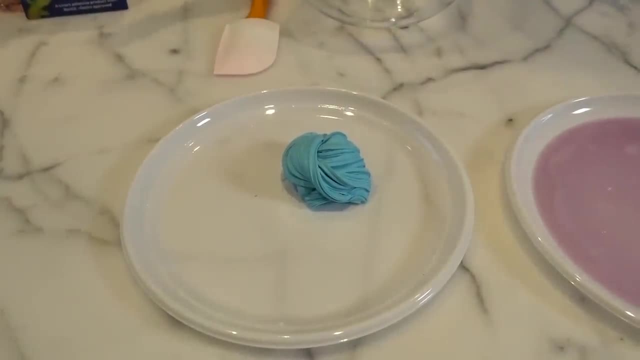 Oops, Alright, guys, I couldn't resist. I had to add colour to my Blu-Tack slime And look, it looks pretty nice. now, actually, I like the colour. Okay, guys, we're on to our very last. no glue or Borax slime, which is cornflour. I'm going. 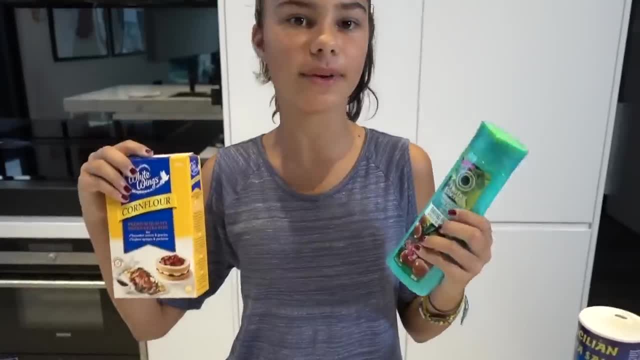 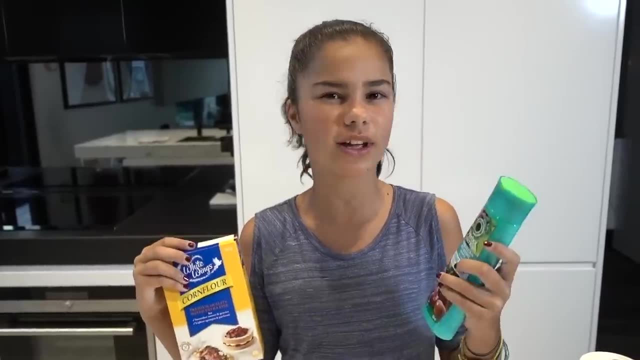 to add in a little bit of lotion, Cornflour and shampoo slime. So when I add some shampoo to the bowl, I'm going to add some cornflour to it as well, And then when I mix it, it's supposed to turn into a buttery. 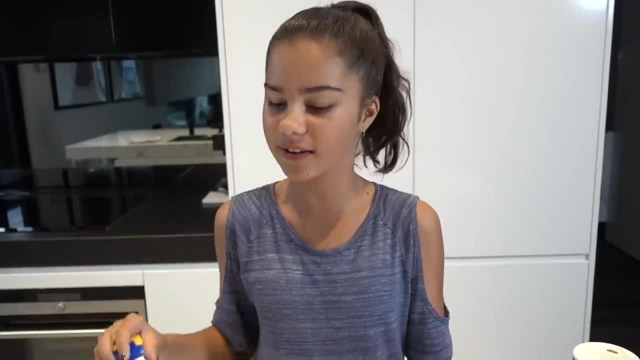 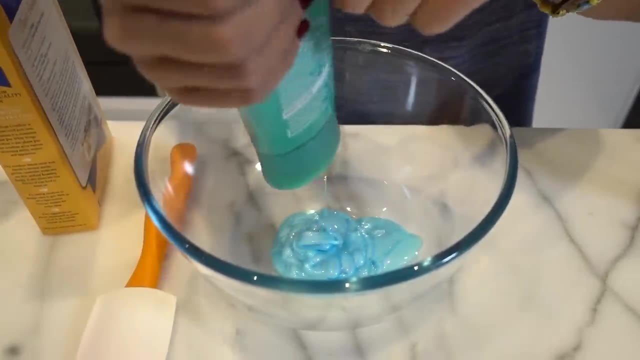 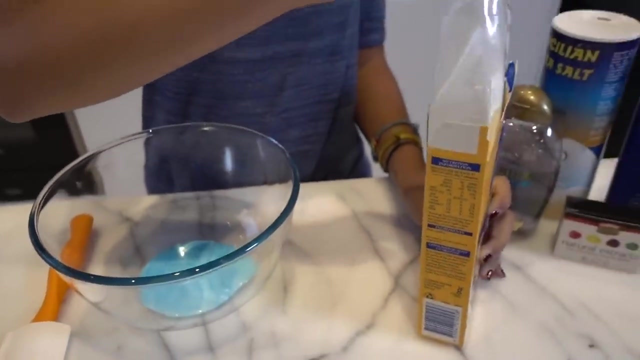 kind of slime, but also really stretchy. So let's see how this one turns out. I'm going to add in maybe that much. Oh, that's probably too much. Oh well, And here I've got my cornflour. 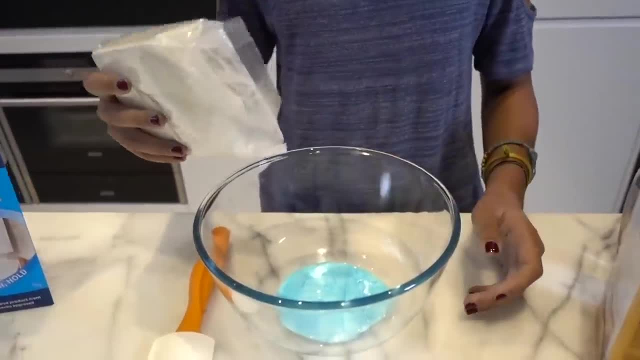 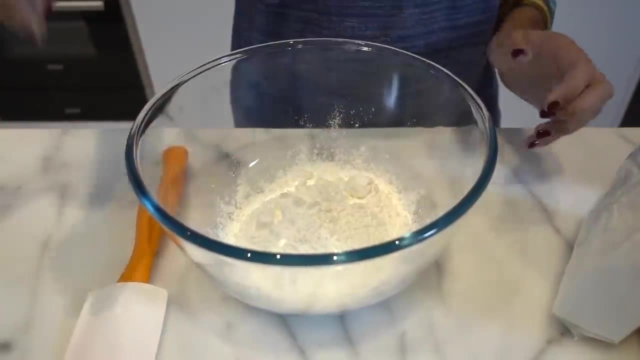 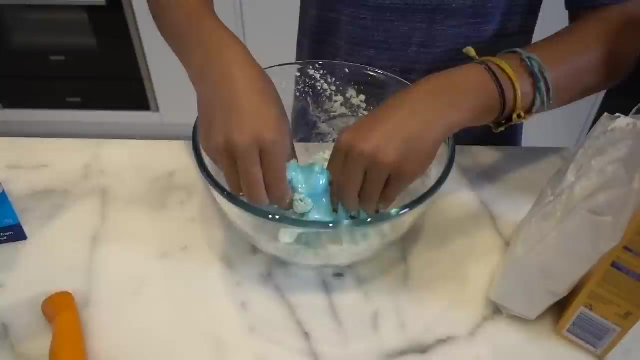 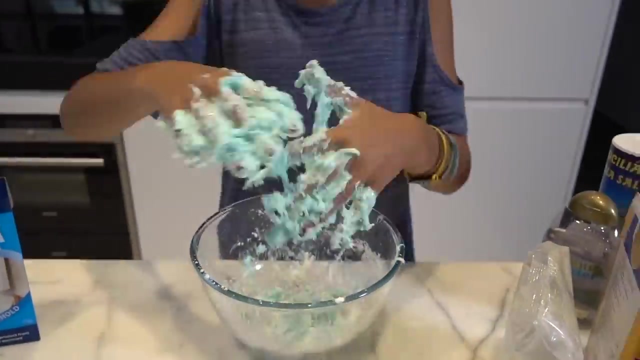 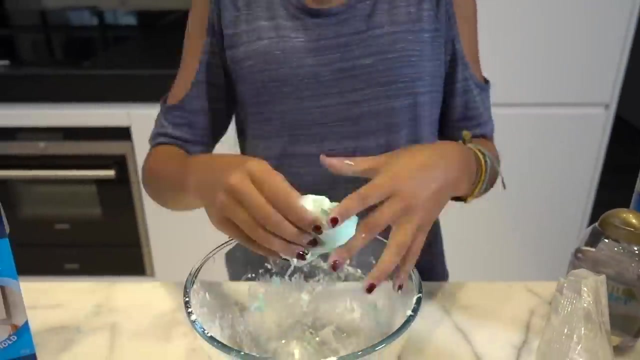 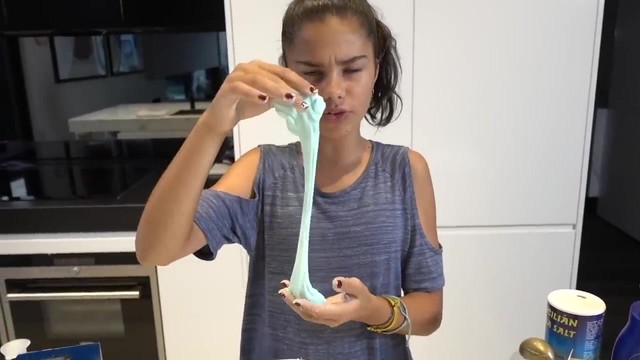 And I'm just going to add maybe about the same amount And let's mix this together. Okay, guys. so after a bit of kneading, this one actually looks like a pretty good slime. I mean, it's got a little bit of texture to it. 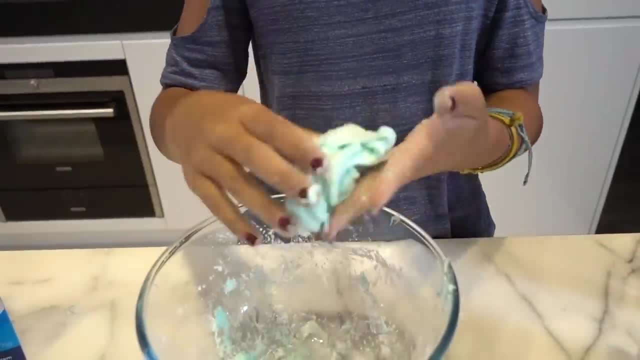 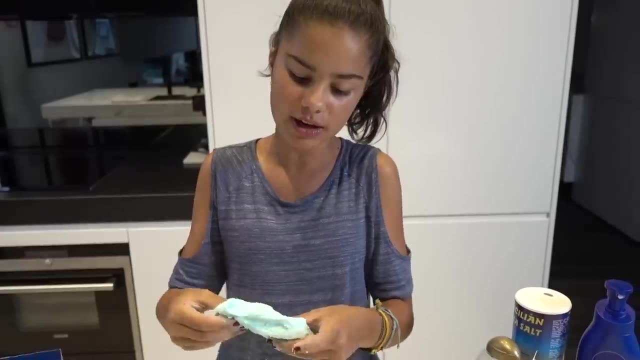 It took a lot of kneading and it turned into a very hot mess and like it was very sticky, I had to try and get it all off my hands. but now, playing with it, it feels really nice, actually, Like it's quite stretchy as well. 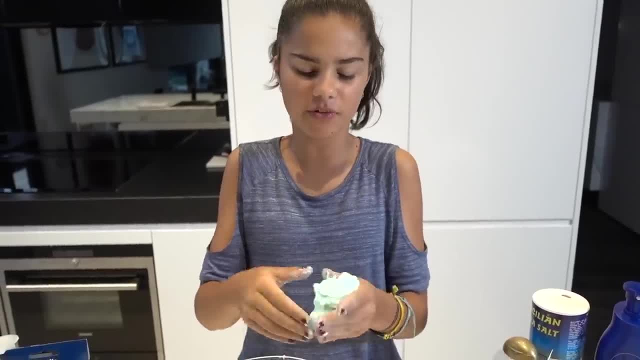 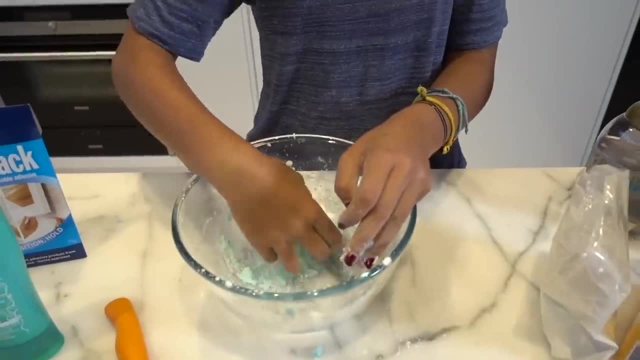 It's a little bit sticky, but that's fine. but it's not, it's very. it's very like buttery and doughy, but it's not very like prickable. Yeah, that's not very good, but anyway it's a pretty good texture, so I'd probably give. 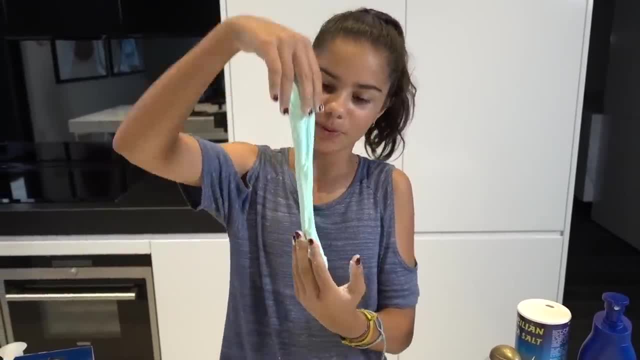 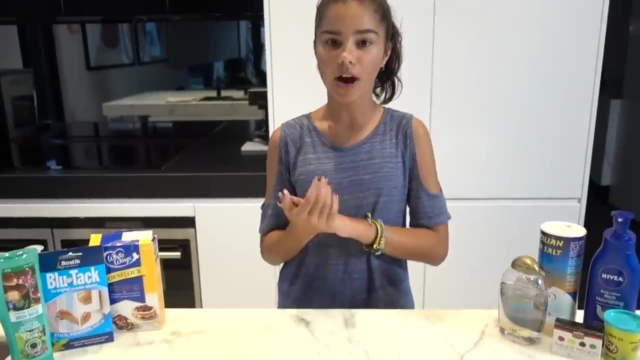 this one a thumbs up. I really like this one. Okay, All right guys. that's four slimes without any glue or borax. I have to say it was actually a lot of fun to make, and my favorite one was probably the Blu-Tack slime. 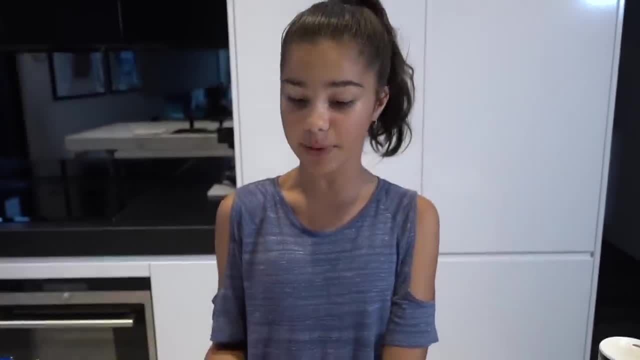 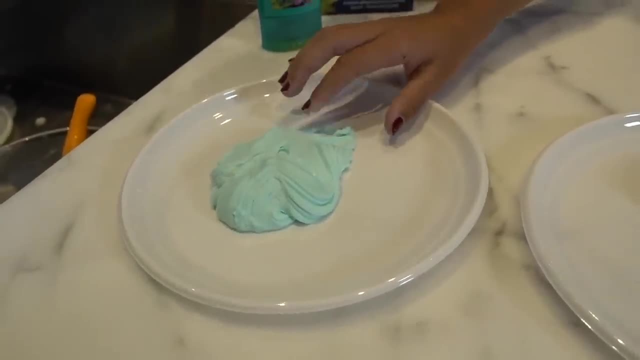 I mean it was really soft and stretchy and it was a lot of fun to play with. but not far behind that was probably the conditioner and cornflour slime. It had a really nice texture and it's also a lot of fun to play with. 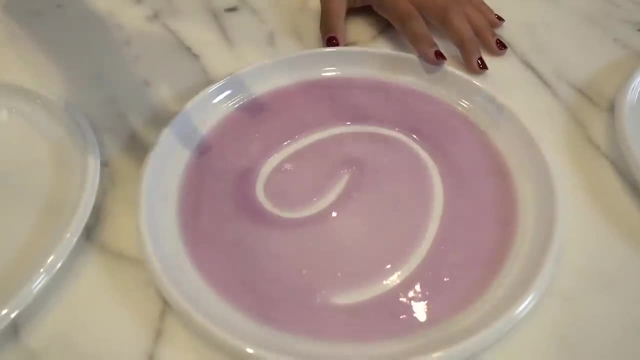 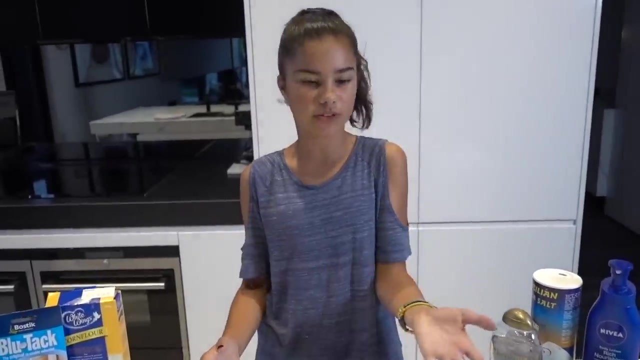 And this one here was definitely the biggest fail, because it is a bit good. Okay, It's not very fun to play with, as you guys can see, and it just didn't work out. Again, if you guys know how to make this one work, don't forget to comment that down below. 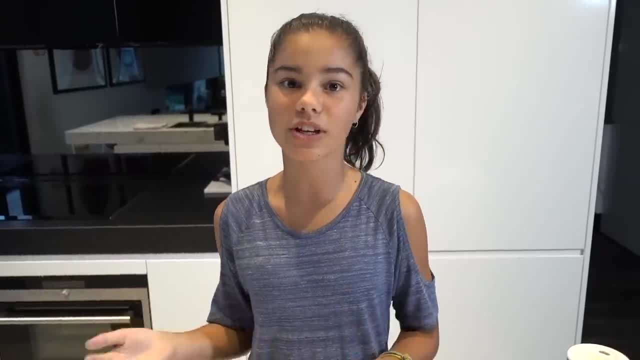 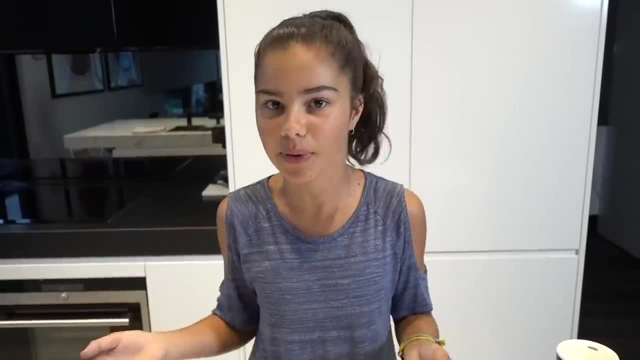 And that's all for this video. I mean, it was really nice to know that you can actually make slimes without glue and borax and with stuff that you have like everyday items, like things around the house as well. So, yeah, I hope you guys enjoyed this video. 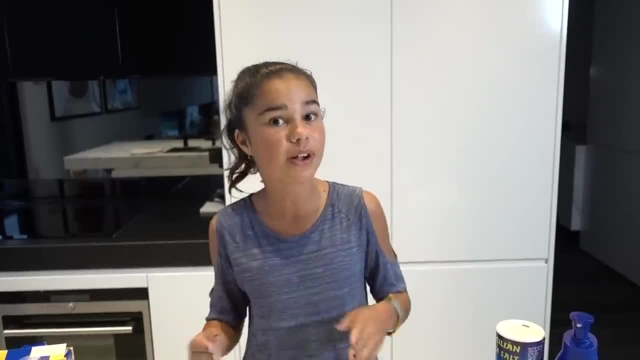 Don't forget to subscribe to my YouTube channel, And also don't forget to check out my Instagram. I'll see you in the next one. Bye, Bye, Bye, Bye. Okay, I've just gotten a new Instagram account, Grace's World Official, and I'll see you.